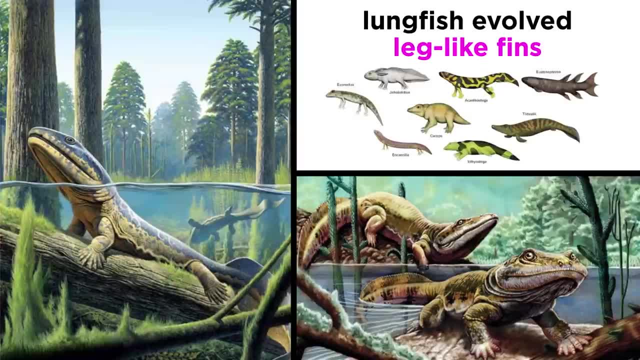 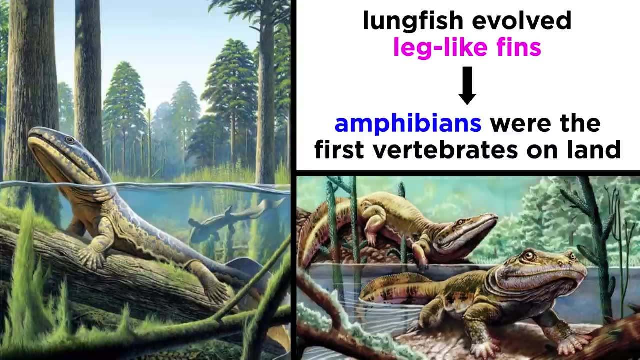 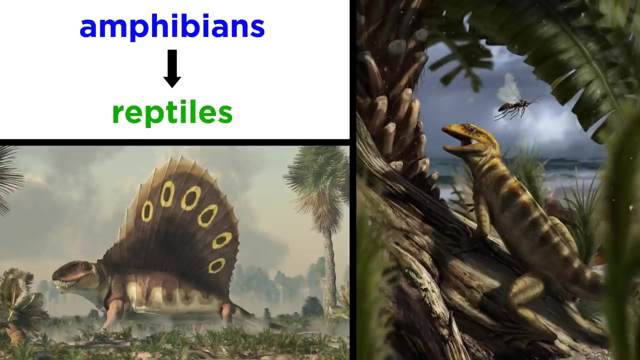 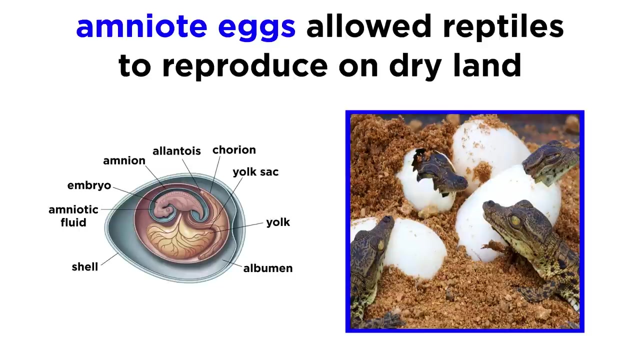 Land plants laid the foundation for brand new ecosystems, as other organisms moved into forests looking for food and shelter, the most consequential being a population of lungfish that evolved leg-like fins. These new animals, amphibians, were the first vertebrates to walk on land. All vertebrates, from dinosaurs to humans, share a common ancestor with amphibians. Before long the land was colonized by amphibians, which evolved into a new species called the reptiles, which evolved into reptiles near the end of the Paleozoic. The main innovation that marks the evolution of amphibians to reptiles was the rise of the amniote egg. 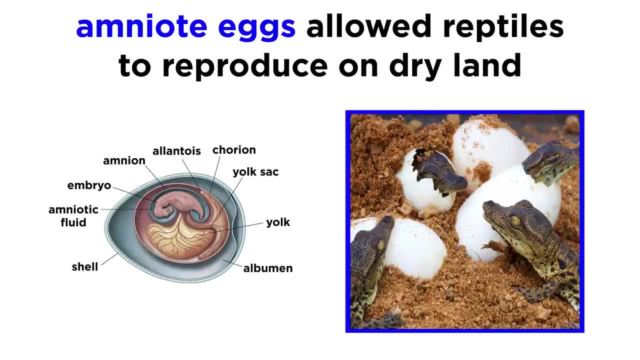 It allowed reptiles to reproduce on dry land, whereas amphibians must return to water for this part of their life cycle. 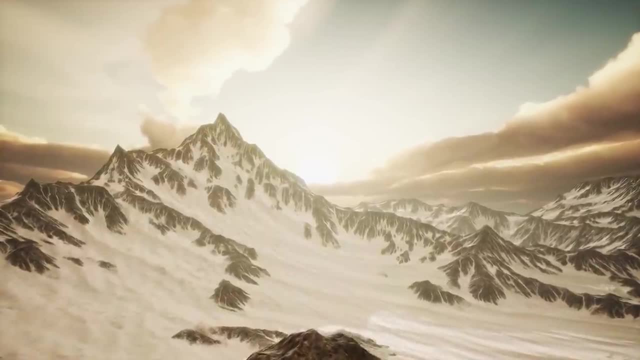 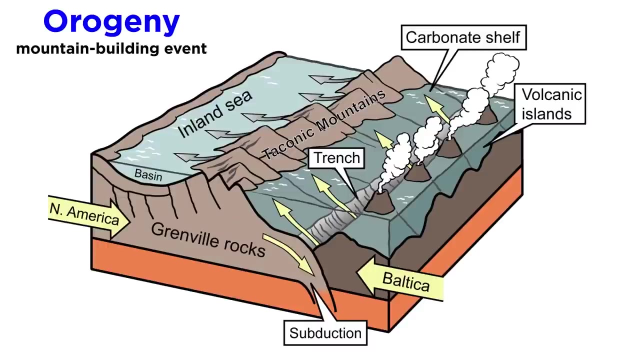 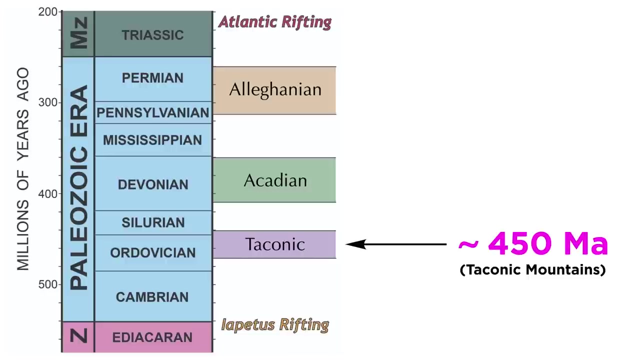 The Paleozoic was a time of great mountain building along eastern North America. North America collided with three separate land masses. Causing three separate orogenies, or mountain building events. The first orogany is called the Taconic Orogeny, occurring 450 million years ago. The second is called the Acadian Orogeny, at 380 million. And the third and final orogany called the Alleghenian Orogeny, occurred 300 million years ago and was responsible for forming the Appalachian Mountains. These mountains were around the size of the Higgs boson. 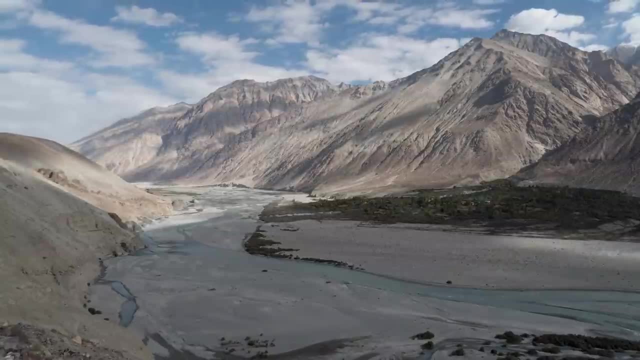 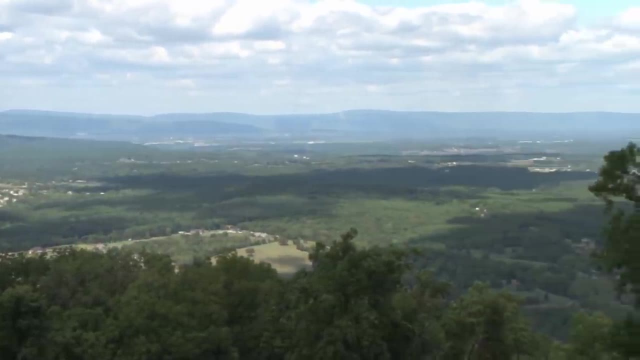 They formed the Himalayas when they first formed, and have extensively eroded over the past 300 million years, leaving behind the resistant stumps of a once great mountain range. 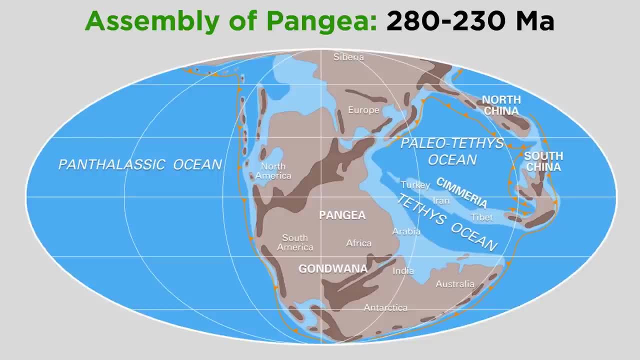 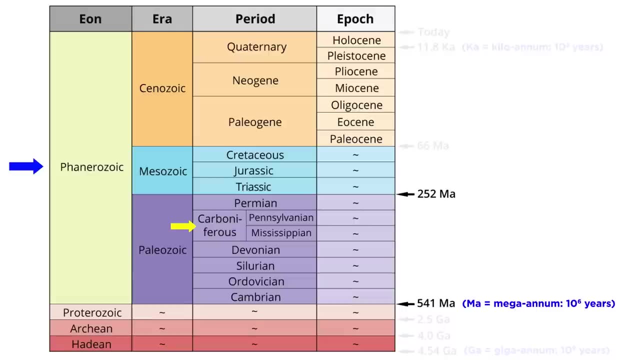 The Alleghenian Orogeny concluded with the assembly of the supercontinent Pangaea at the end of the Paleozoic. An important geologic period toward the end of the Paleozoic era is called the Carboniferous Period. 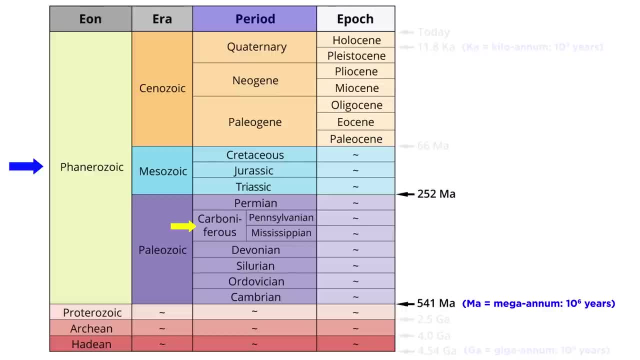 A geologic period is a more specific classification of geologic times. A geologic period is a more specific classification of geologic times. A geologic period is a more specific classification of geologic times. 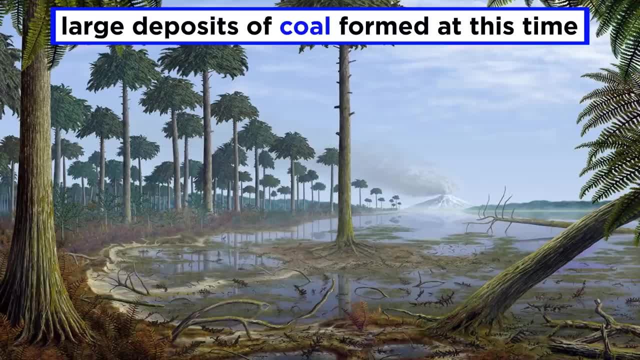 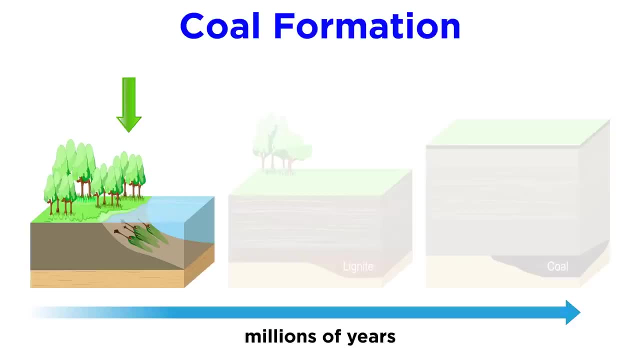 The Carboniferous Period is named for the large deposits of coal that were formed during this time, deposits that span the entire globe. The Carboniferous Period is named for the large deposits of coal that were formed during this time, deposits that span the entire globe. Coal forms when plant tissues are rapidly buried in anoxic conditions in coastal and inland swamps. 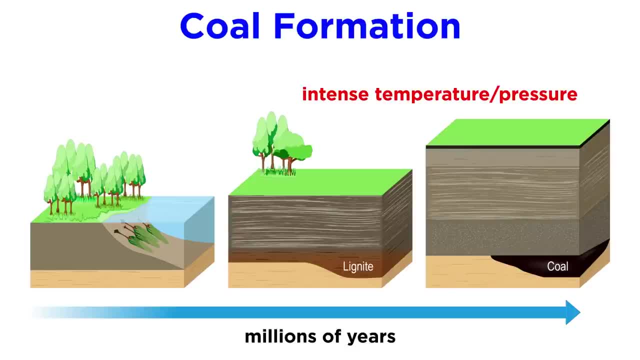 Rapid burial of organic material requires rapid fluctuations in sea level, which are caused by the formation and melting of glaciers. So, without a geologic period, there is no geologic period. So, without a geologic period, there is no geologic period. 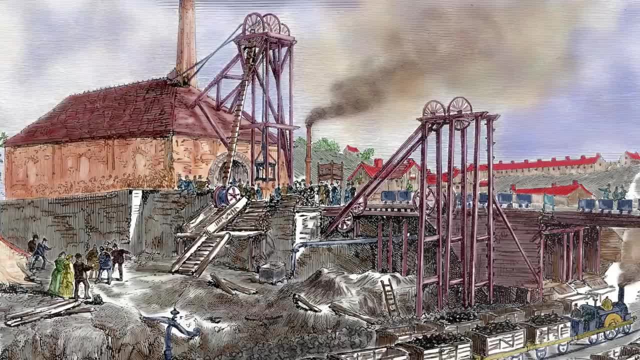 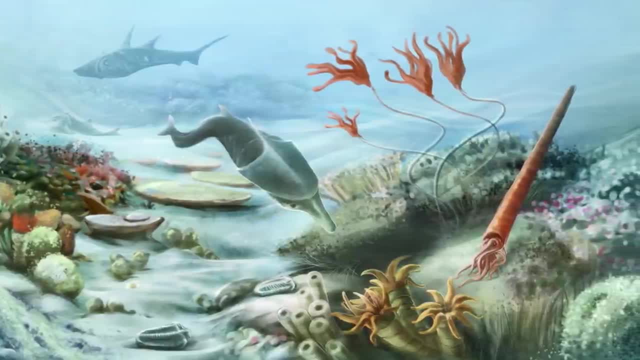 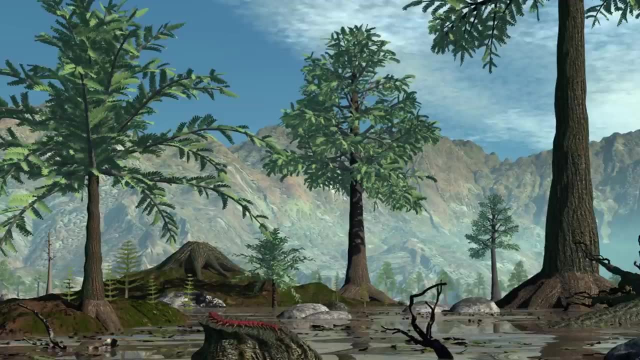 So, without carboniferous glaciers, the industrial revolution may not have occurred. In summary, the Paleozoic era was a time of dramatic transformation, for both the Earth and its inhabitants, so it seems only fitting that the era would go out with a bang. 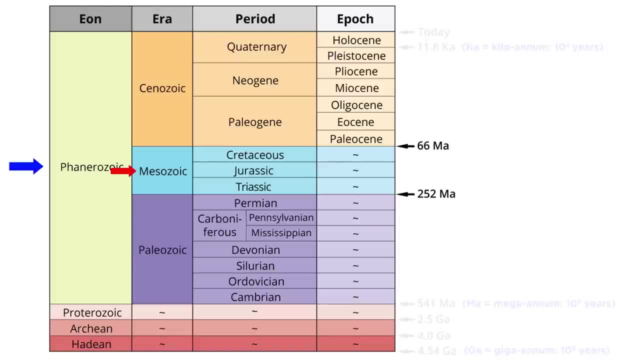 Let's move forward and find out precisely what happened to prompt the next era of the Phanerozoic Eon. 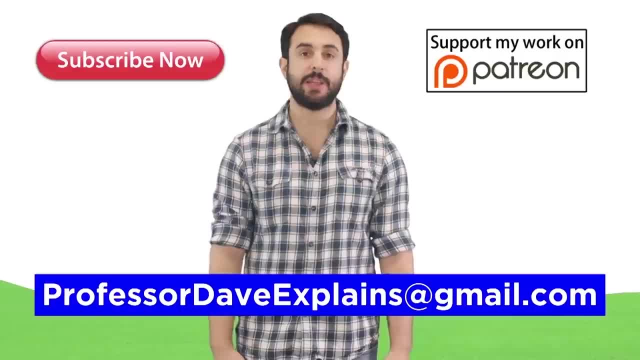 Support me on Patreon so I can keep making content, and as always, feel free to email me, professordaveexplains at gmail dot com. 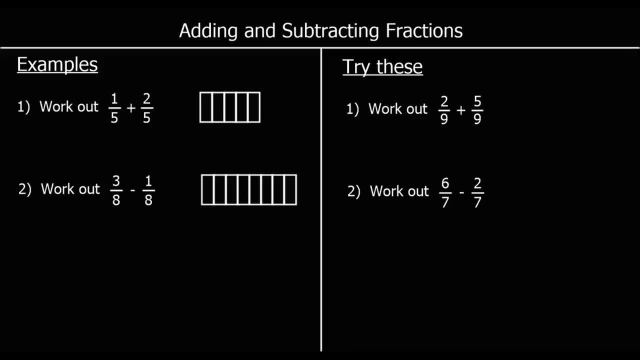 We can only add things that are the same. With fractions, that means we can only add fractions with the same denominator, with the same number on the bottom. So we can add thirds to thirds, or quarters to quarters, or fifths to fifths, or sixths to sixths, and so on. So we can only add them when they are the same. The first question says, work out one-fifth plus two-fifths. So if we've got one-fifth of something, one-fifth of this shape, and we add two-fifths, so one part plus two parts, means we've got three parts. 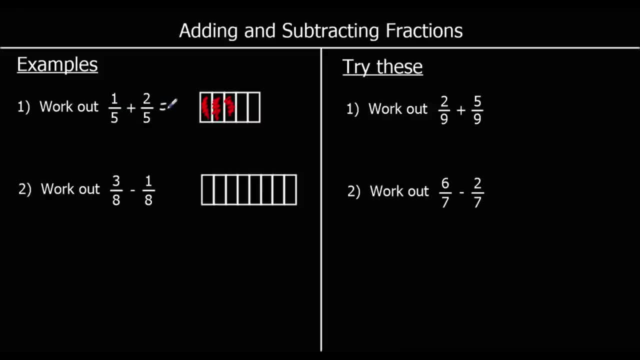 So one-fifth plus two-fifths is three-fifths. And taking away is the same. So we can only take away fractions with the same denominator. 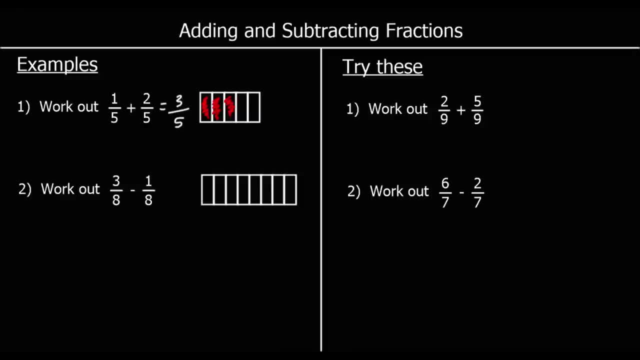 So we've got three-eighths, take away one-eighth. So if we've got three parts, and we take away one part, that means we've got two parts. So three-eighths, take away one-eighth, is two-eighths. Two-eighths.